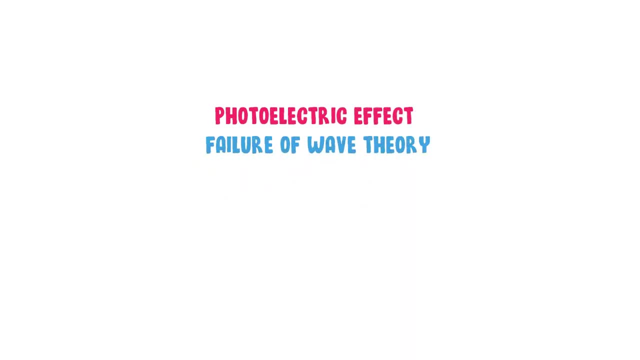 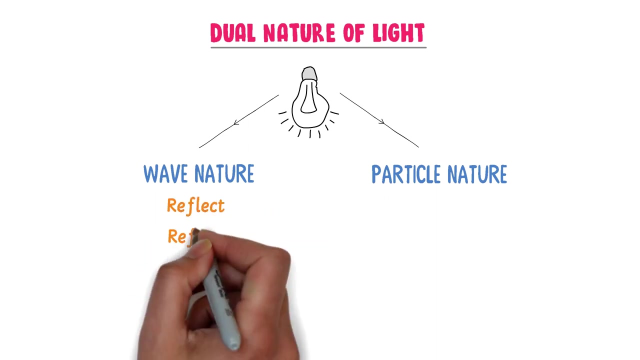 Photoelectric effect, failure of wave theory and how Einstein's photon theory explained it successfully. We have learned in the previous lecture of dual nature of light that light has wave nature and particle nature. Light reflects refracts and diffracts, so it has 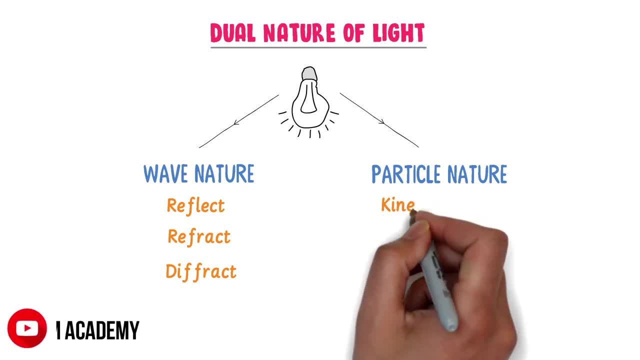 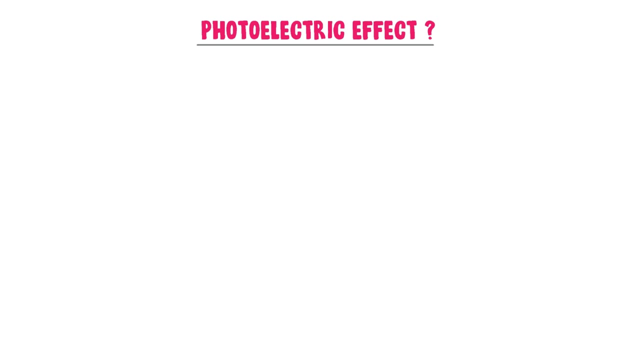 a wave nature. Secondly, light transfer kinetic energy and momentum to electron, so it has particle nature. Therefore we say that light has Archeri's nature of wave and particle. Now, what is photoelectric effect? Well, consider a metal surface. I incident red light on this. 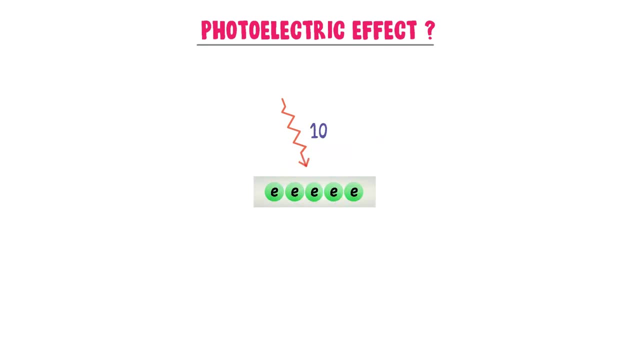 metal surface. Let the frequency of red light is 10 to the power 14 hertz. We know that light is made up of photons. Now consider this moving photon Due to its motion. this motion is made up of photons. Now consider this moving photon Due to its motion. 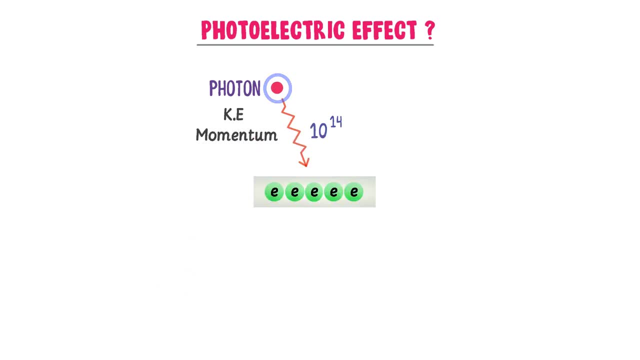 this photon possesses kinetic energy and momentum. When this moving photon hits the electron of the metal surface, it will transfer its momentum and kinetic energy to this electron. As a result of this collision, electron will be ejected from the metal surface. Thus we 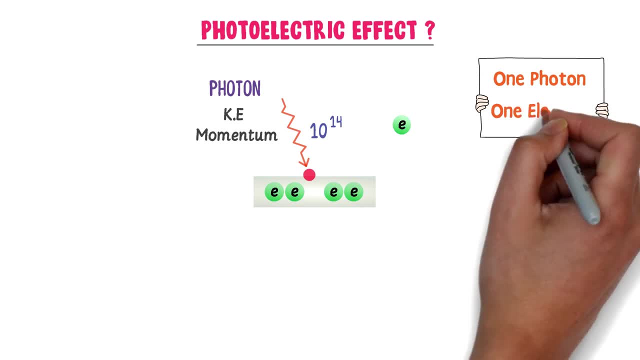 can see that one photon of red light ejects one electron from the metal surface. Let me repeat it: One photon of red light ejects one electron from the metal surface. Let me repeat it: One electron of red light ejects one electron from the metal surface. Thus, 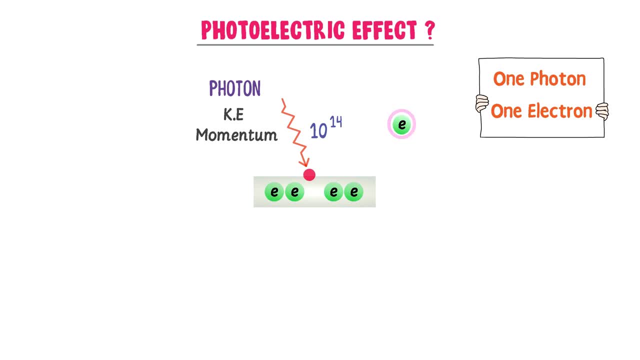 we can see that one electron of red light ejects one electron from the metal surface. Remember that this ejected electron is called photoelectron, because they are ejected by the photons of light. Now, if we provide a conducting path to these photoelectrons, they will move. 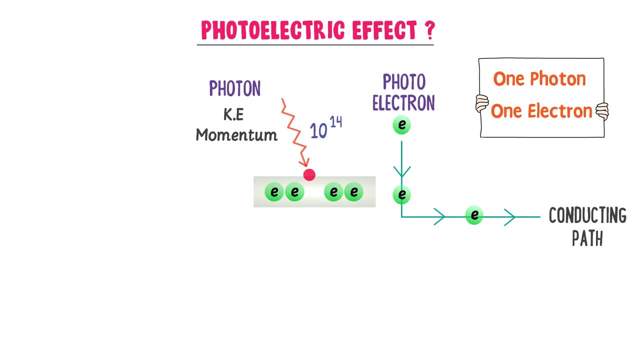 from high potential region to low potential region. These photoelectrons are moving, so they produce current, which is called photoelectric current. Therefore, we define photoelectron effect as the phenomena in which electrons are ejected from a material after absorbing a suitable frequency. Let me repeat it: The phenomena in which electrons are ejected from. 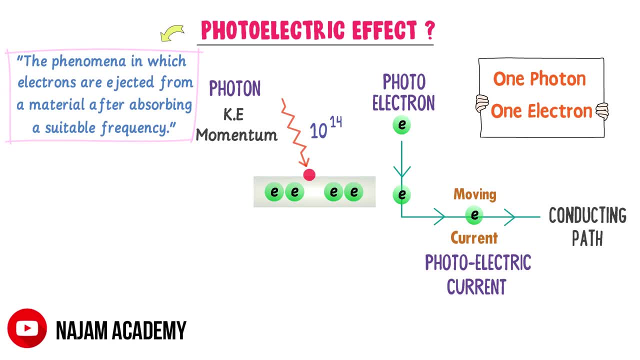 a material after absorbing a suitable frequency. Here let me teach you one important question: Does every light eject electron from metal surface? Well, the answer is no. Not every light ejects electron from metal surface. Here let me teach you one important question. 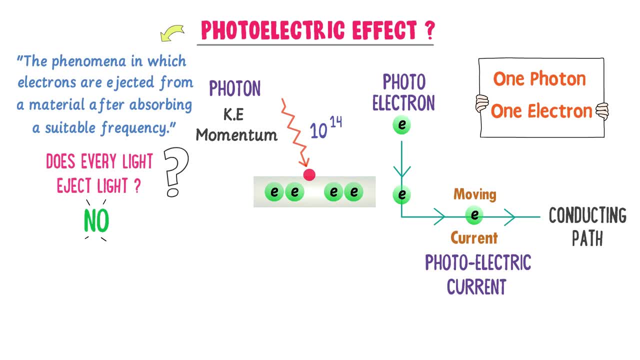 ejects electron from the metal surface. Do you understand threshold frequency? Well, threshold frequency means minimum frequency of an incident light to eject electron from the metal surface. For example, the threshold frequency needed to eject this electron from metal surface is 10 to the power 14 Hz. 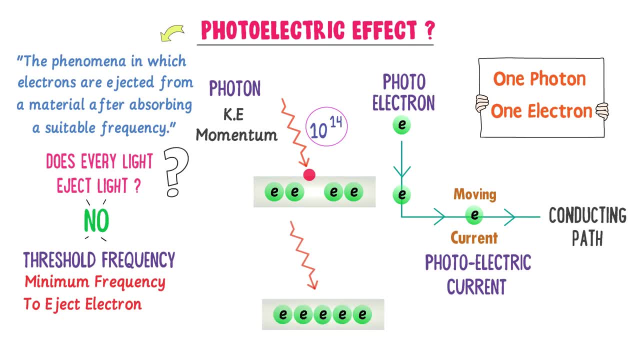 If you incident light, a frequency less than 10 to the power 14 Hz, like 10 to the power 8 Hz, it will not eject electron. Also, you should learn that what would happen if the threshold frequency is exceeded? Well, the electron would be ejected and it will move with greater speed, or its kinetic. 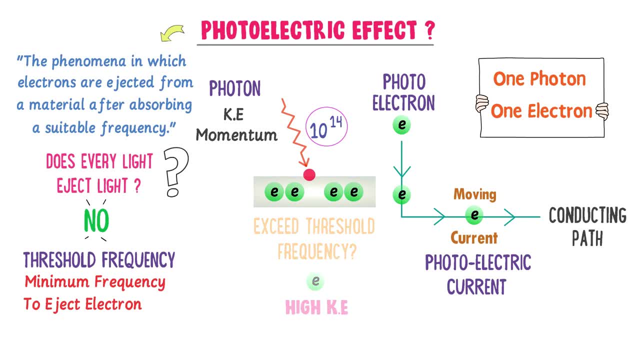 energy will be high. Secondly, you should also understand work function. We define work function as work function. The minimum energy needed to remove an electron from a metal surface is called work function. So until now, we learned about photoelectric effect, a phenomena in which electron is ejected. 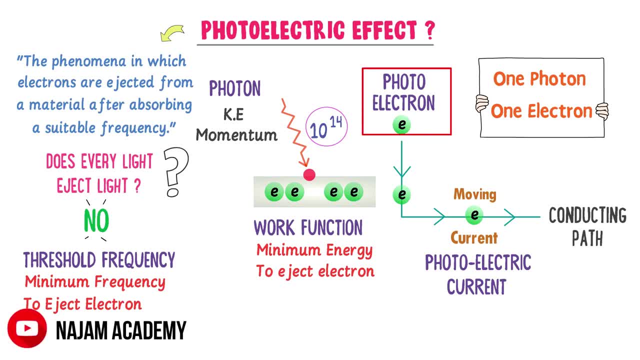 by photon Photoelectrons. electrons released from metal surface due to incident photon Photoelectric current. when photoelectron starts moving, the minimum energy needed to remove an electron from metal surface is called work function. The threshold frequency: the minimum frequency required to remove an electron from metal. 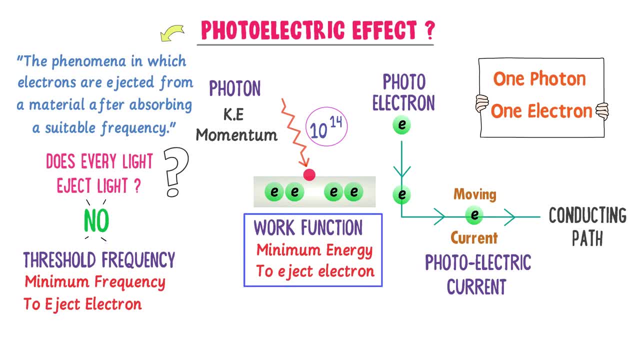 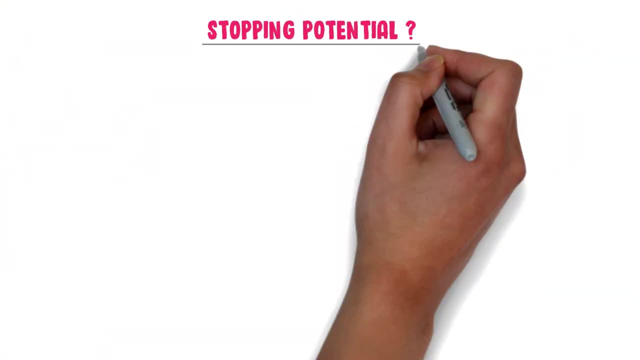 surface work function, the minimum energy needed to eject an electron from metal surface, etc. So note it down, all these important terms related to photoelectric effect. Now let me teach you the concept of stopping potential, For example. consider this system, in which one metal plate is connected to positive termination. 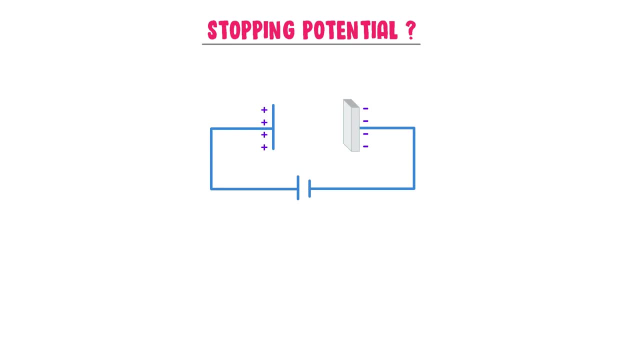 For example, consider this system in which one metal plate is connected to positive termination, So where one is connected to the negative terminal of the battery and another is connected to the negative terminal of the battery. so this battery has potential difference of 20 volts. so I use I rather 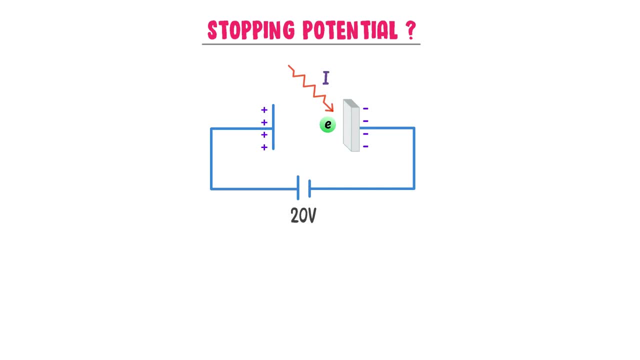 I, In this case I incident red light of intensity I on this divide. As a result, electrons will be ejected from the metal surface and these photoelectrons would be attracted by the positive plate and this ammeter would be deflected to indicate. 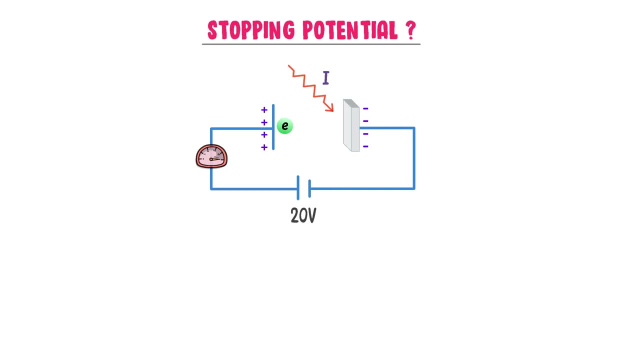 the flow of photoelectric current and their electric current. 뭘 I can I use here? My current plants are screw. this current próp master is a right one for me- calculator. Should I turn this into a current If I show this set of square tubes like this? 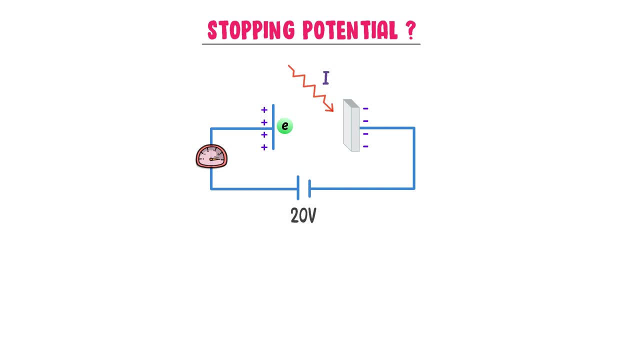 The plate is here. Here the circuit To create relationship between photoelectric current and voltage. let me draw a graph. I take voltage along x-axis and photoelectric current along y-axis. We know that a 20V maximum current is produced. 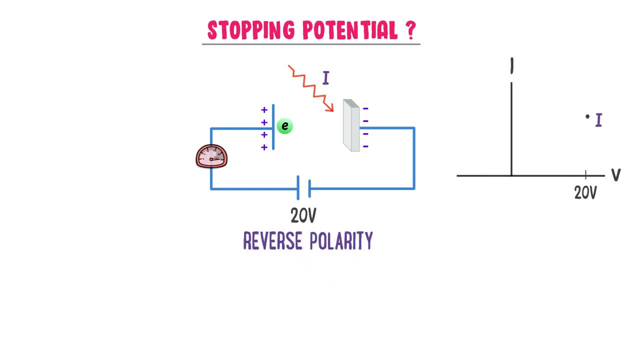 Now listen carefully. I reverse the polarity of a battery. I mean shifting terminals are connecting the plates to opposite terminal of the battery. By reversing polarity, this plate will become negatively charged and this negative plate will become positively charged. The voltage of the battery is considered minus 20V due to reverse polarity. 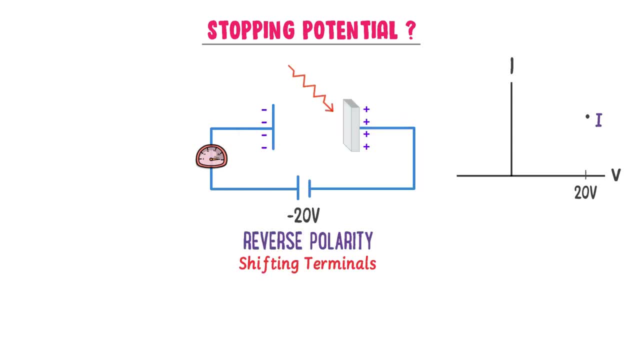 Now, if I incident red light on the metal surface, it will eject electron, but this electron will not reach to this negative plate because both have light charges And they repel each other. So we say that minus 20V is called stopping potential because it stopped this electron from reaching to this plate. 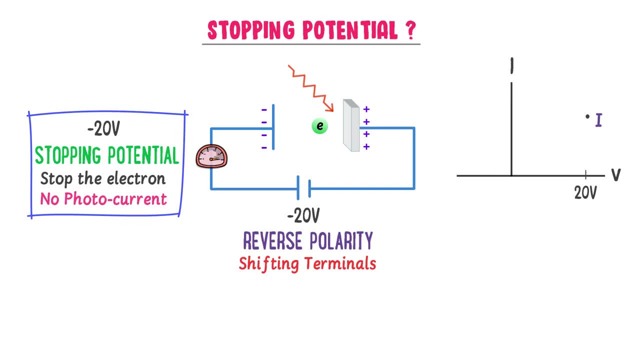 Let me repeat it: minus 20V is called stopping potential, because it stopped this electron from reaching to this plate. We know that a 20V maximum current is produced, but when we reverse polarity At minus 20 volt, no photoelectric current is produced. 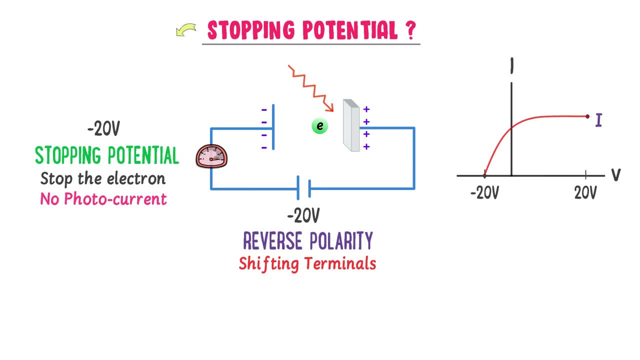 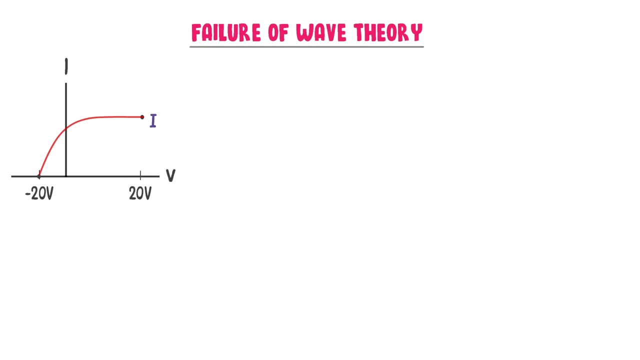 So the graph becomes like this. Therefore, we define stopping potential as the minimum potential required to stop electrons from moving between plates is called stopping potential. Thus, note it down that stopping potential stops the electrons between plates. Now we are going to learn the failure of wave theory to explain photoelectric effect and 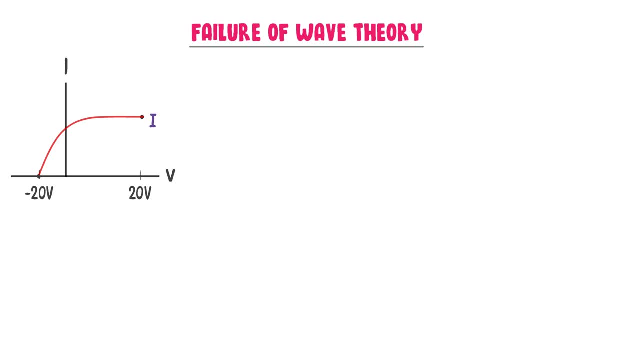 stopping potential. We have already learned that at 20 volt maximum photoelectric current is produced, While at minus 20 volt no photoelectric current is produced or it is the stopping potential. In old period or classical period, scientists were interested that at minus 20 volt this 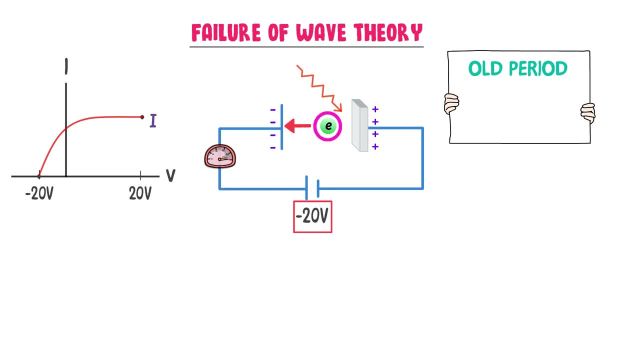 photoelectron should stop. Should it stop should reach to this plate, But how it would be possible? Well, it will reach to this plate if the kinetic energy of the photoelectron is increased. They stated that kinetic energy of the photoelectron is directly proportional to the intensity I of the incident light. 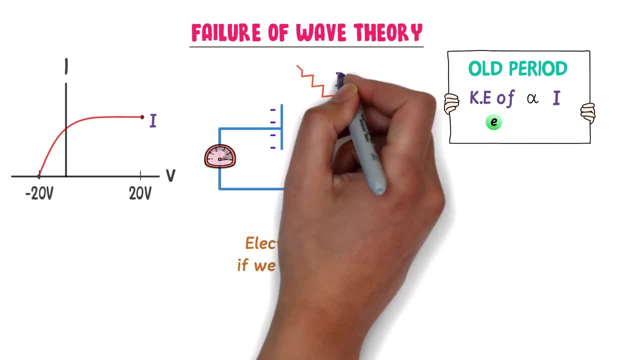 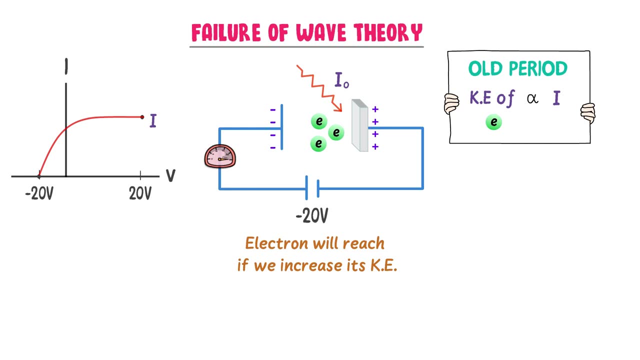 Hence they increased the intensity of the red light to I0. But they saw something strange. The red light of intensity I0 ejected these electrons, but they didn't reach to the plate. So the stopping potential is still minus 20 volt. So their logic was wrong, that kinetic. 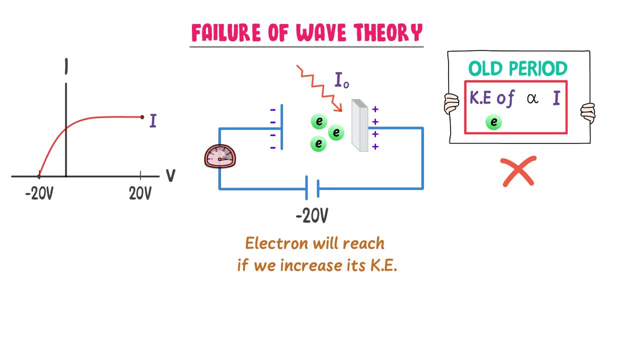 energy of the photon is directly proportional to the intensity I of the incident light, Because the higher intensity red light didn't increase the kinetic energy of these photoelectrons. rather, higher intensity of red light didn't increase the kinetic energy of these photoelectrons. 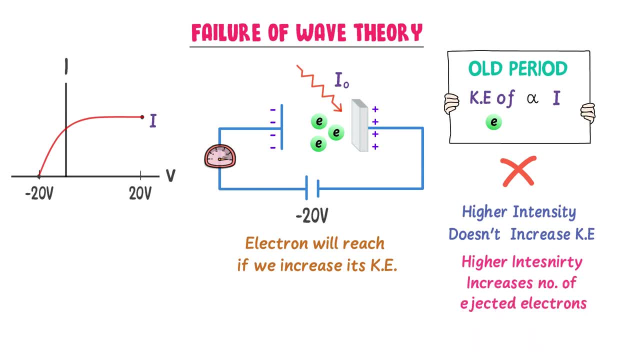 Red light only increased the number of ejected electrons, So we get this type of graph where stopping potential is still minus 20 volt. Hence this was the big problem, that why increasing intensity of light doesn't increase the kinetic energy of photoelectrons. 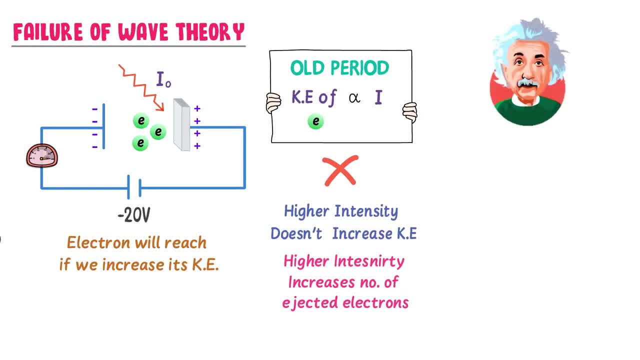 Well, here comes Einstein Baba. He successfully explained and solved this problem by presenting his famous photon theory. He stated that kinetic energy of the emitted electrons depends on the frequency of the incident light, not on its intensity. For example, consider red photons and blue photons. 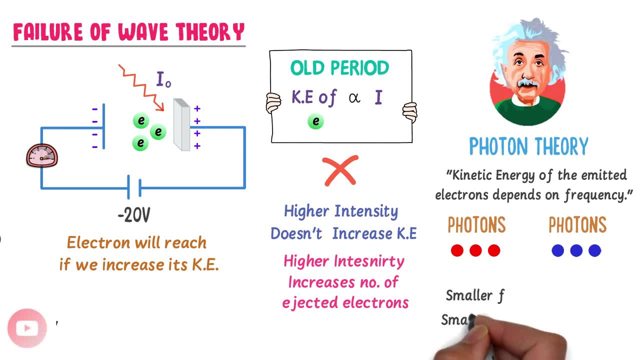 We know that red light has lower frequency, So the kinetic energy of photons would be smaller, While the frequency of the blue light is higher, So the kinetic energy of the photons would be high. For example, red light has lower frequency, So the kinetic energy of the photons would be. 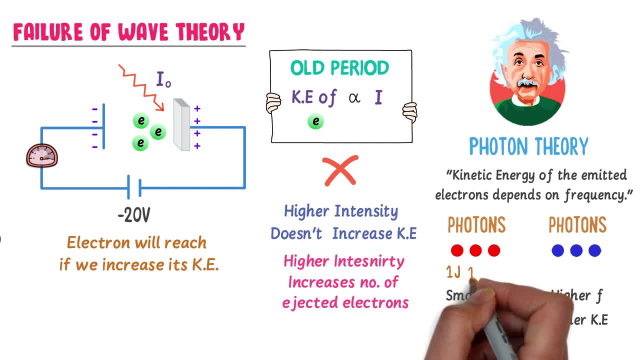 higher. For example, if the kinetic energy of red photons is 1 Joule each, then the kinetic energy of blue photons would be 4 Joule each. That is because the frequency of blue photons is higher than the frequency of red photons. Now, according to Einstein, Baba, if you incident 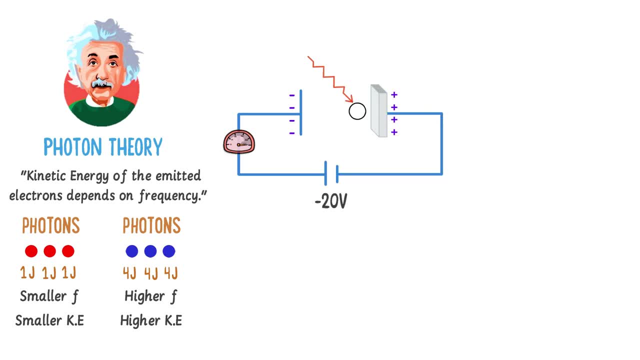 red light on a metal surface, it will eject electron and its kinetic energy would be smaller. So its stopping potential would be minus 20 volt, So the kinetic energy of red photons. But if you incident blue light on the same metal surface, it will eject electron and 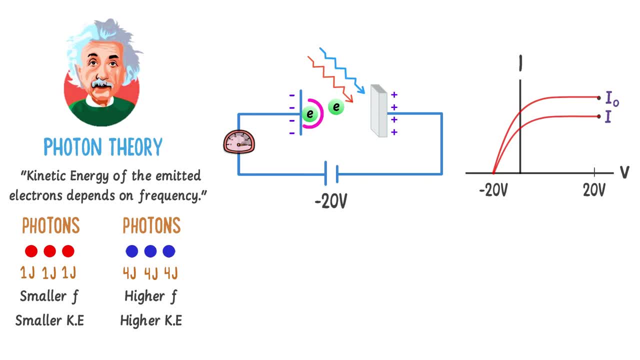 its kinetic energy would be high, so it will easily reach to the plate. It means –20V cannot stop the electron emitted by the blue light. Its stopping potential increases. for example, it may increase to –60V, So we would get this type of graph. 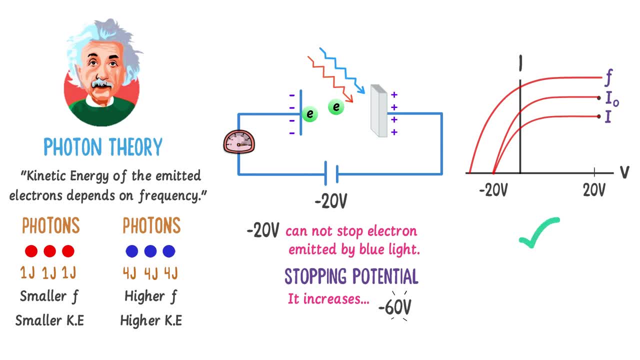 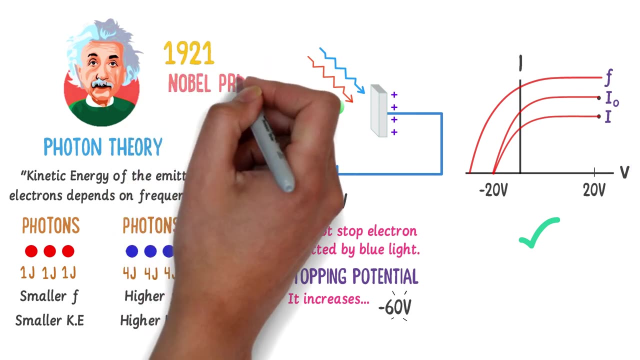 Therefore, Einstein Baba was 100% right that kinetic energy of the emitted electrons do not depend on intensity, rather it depends on frequency of the incident light. For this achievement he was given Nobel Prize in 1921.. I hope that you have learnt all about photoelectric effect. Thank you for watching. 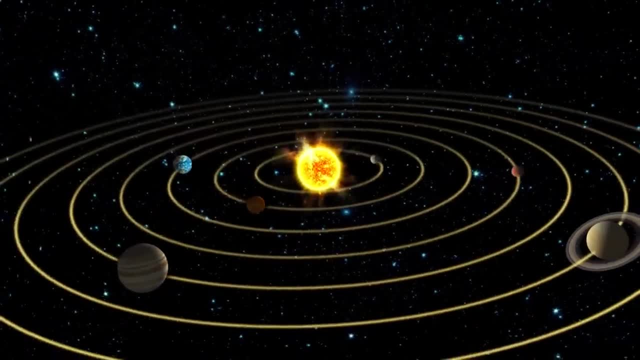 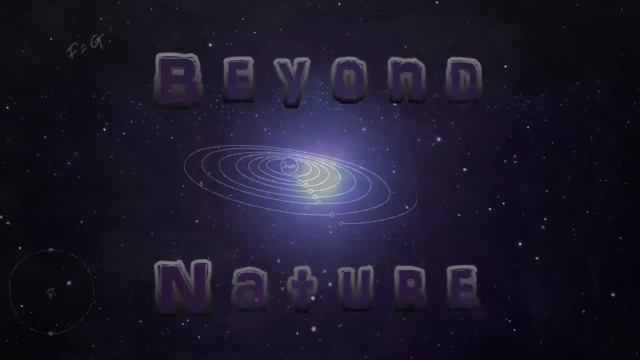 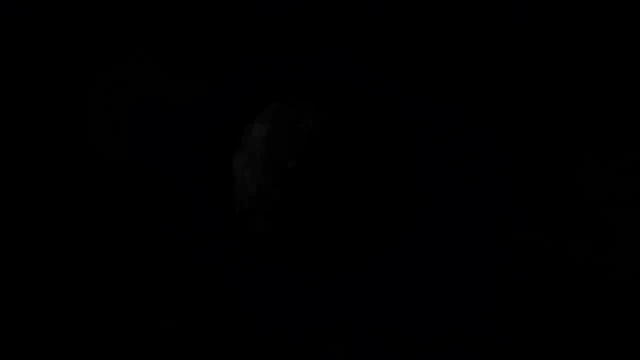 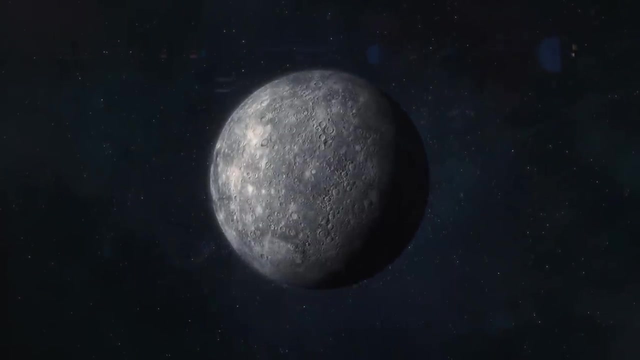 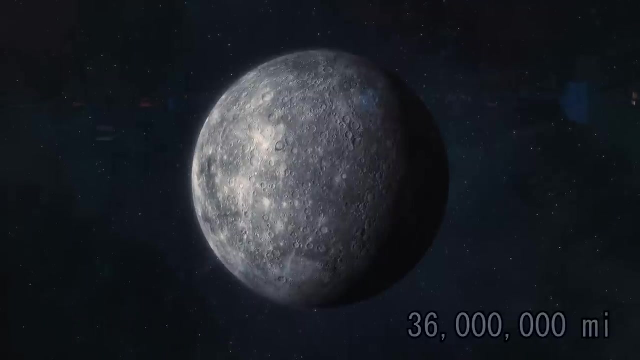 Today, we will explore the planets in our solar system. Thank you for watching. Sit back and enjoy. We will start off with the planet closest to the sun, Mercury. Mercury is a terrestrial or rocky planet that orbits just under 58 million kilometers from the sun, or 36 million miles. 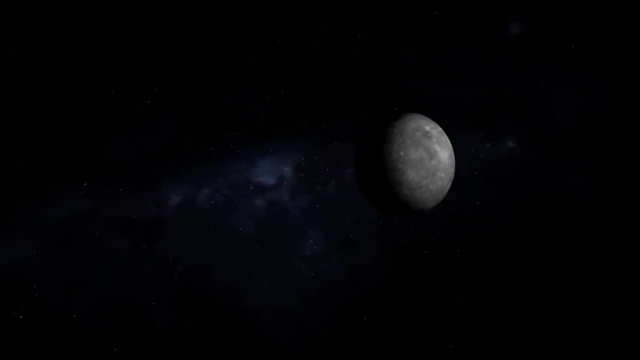 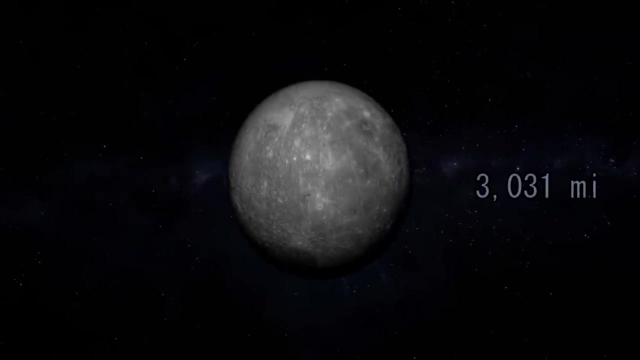 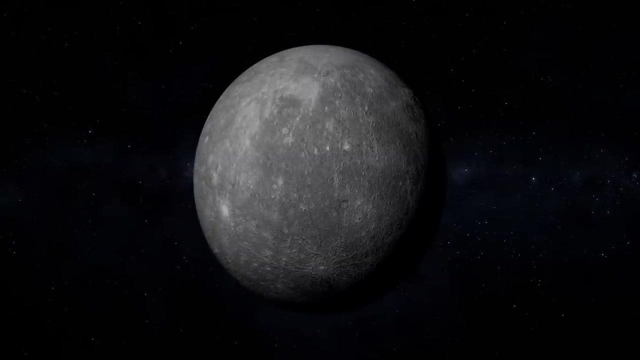 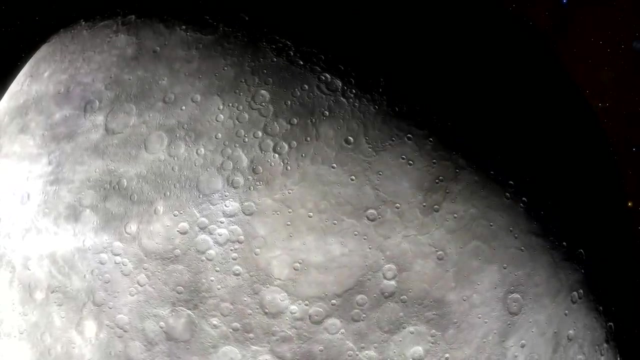 It is the smallest planet in the solar system. with a diameter of just 4,879 kilometers, It is only slightly larger than the Earth's moon, and the two actually look quite similar. Despite Mercury's small size, it is the second most dense planet in the solar system.